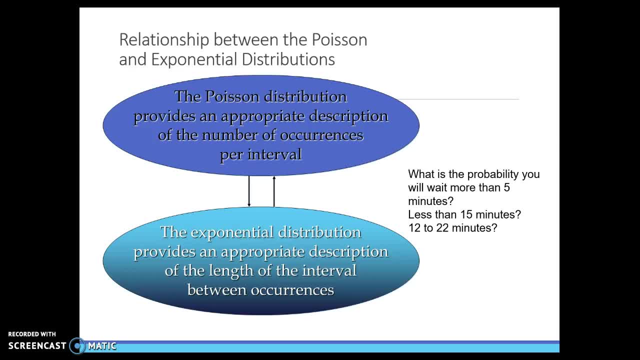 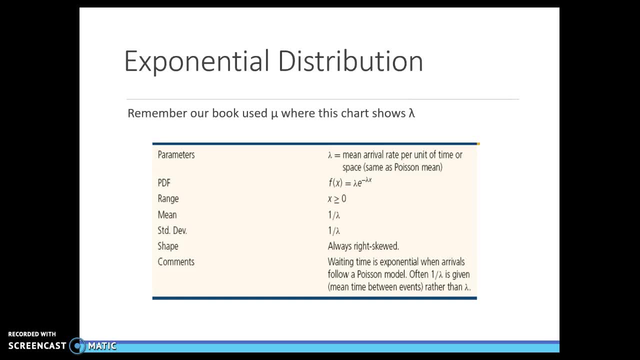 five minutes or less than 15, or 12 to 22 minutes. That's the thing. that's the kind of question that exponential distributions will answer. So our parameters: this is lambda, which in this case lambda, represents the mean arrival rate per unit of time or space. 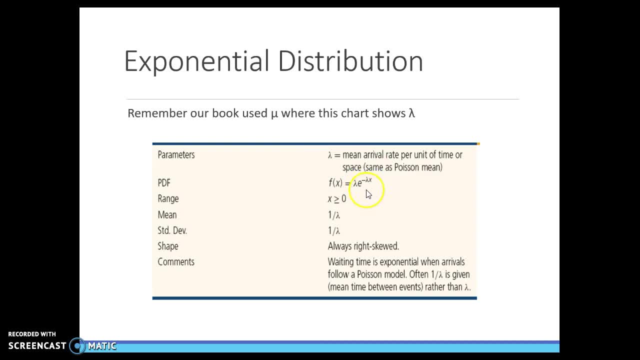 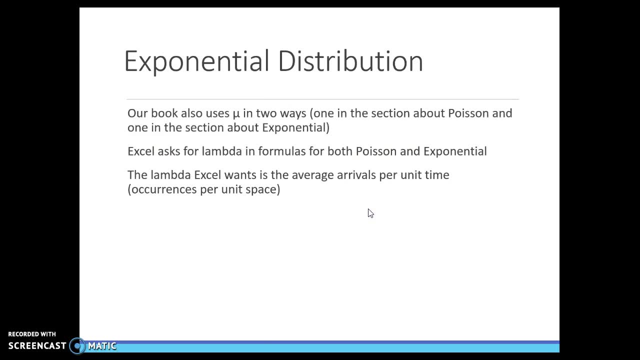 We'll come back to that. The probability distribution function you can see is exponential. Our range is simply above or equal to zero. The lambda that Excel is asking for is the mean time, So it wants the average arrival time per unit of time. It's kind of awkward to think about. Just FYI, some books use mu, some books. 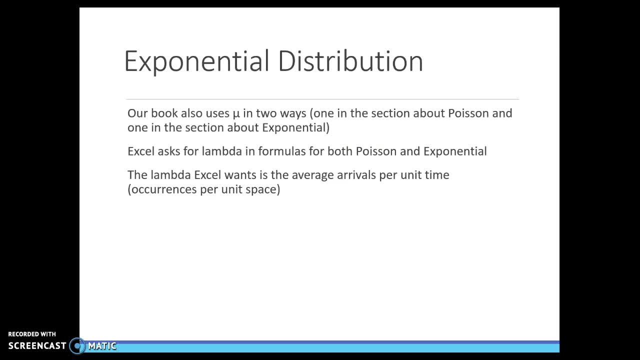 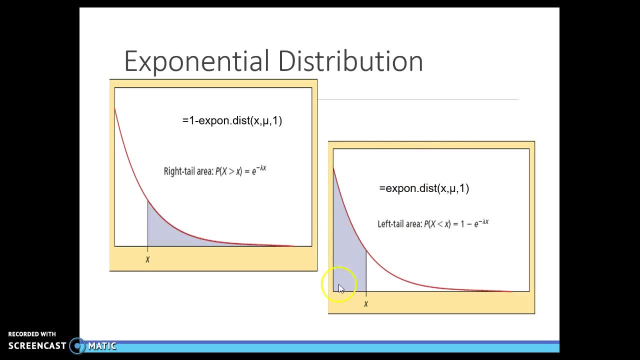 use lambda but they don't use mu, So it's kind of awkward to think about. So it's kind of awkward to think about, But they're essentially talking about. lambda represents the mean of what's expected In Excel. this is your equation, And this equation is assuming that you were interested in up to 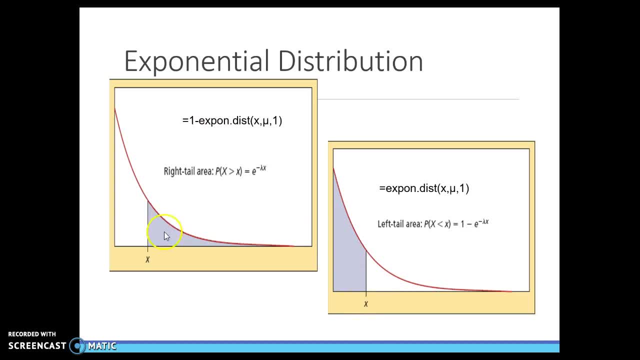